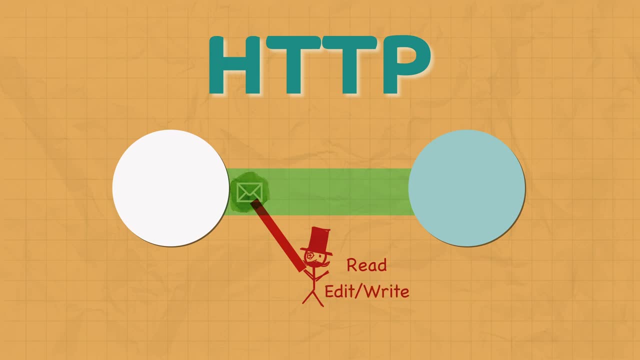 or, in some cases, it can alter the communication between client and server. In any case, this is breach of privacy, of security. A malicious actor or a third party intercepting the communication between two other parties that is expected to be private is also known as man-in-the-middle attack. It is a well-known occurrence in the field of security. 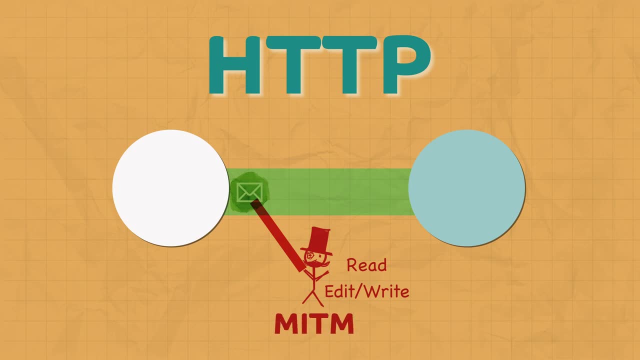 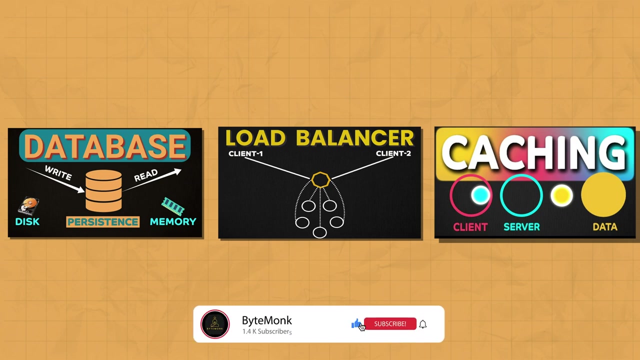 It is usually written by its acronym MITM attack or man-in-the-middle attack. This is, at the core, what we are trying to solve with security. Before moving forward, a quick disclaimer. Unlike most of the other system design concepts like storage, load balancer caching, it is almost certain that you are not required to know much. 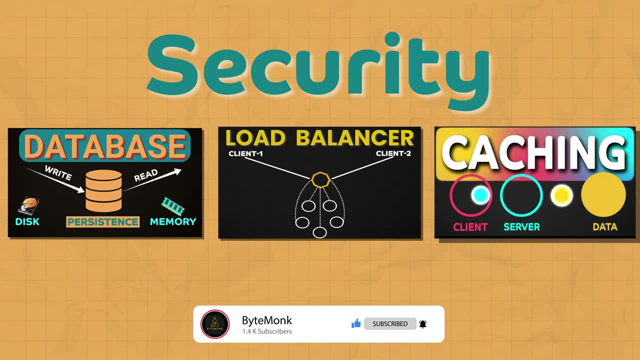 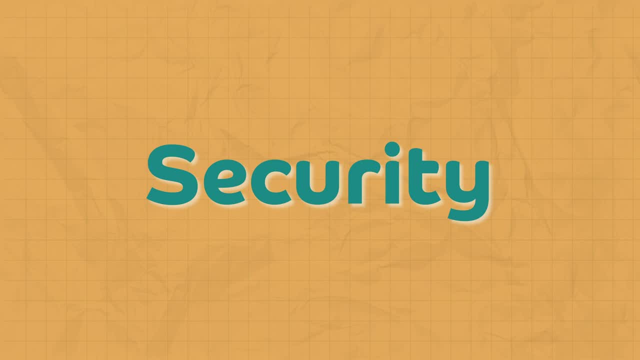 about security. However, it is in your best interest to familiarize yourself with high-level understanding of security, Because system design interviews can go in many directions and it is quite likely that you might start to have a conversation with the interviewers that leads to some topic on security. So having a decent 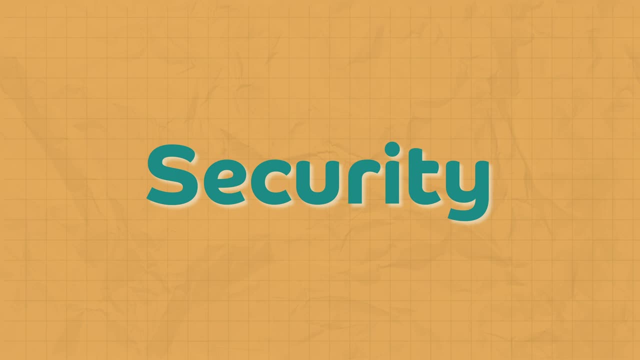 high-level understanding on building blocks of security will help you to confidently design your system. The bottom line for haciendo un webpage is that it would be like to connect to the wireless mily daran or the IP address in your local ACE's, or to wirelessly communicate with the network that provides it another form of the 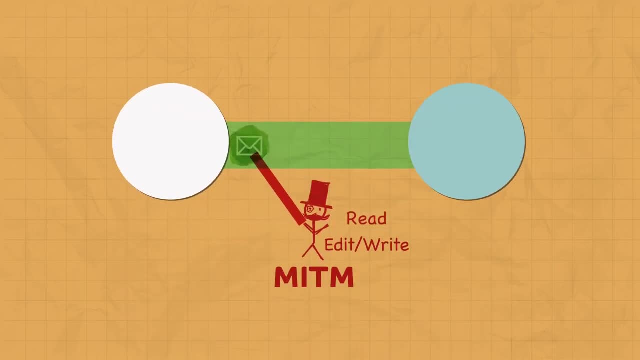 CPU and you would now need that Muslims to do the particular communication with your security. By now you are clear that when you get a client and server communication over HTTP, their communication is not secure. Most of you might have already guessed that we need 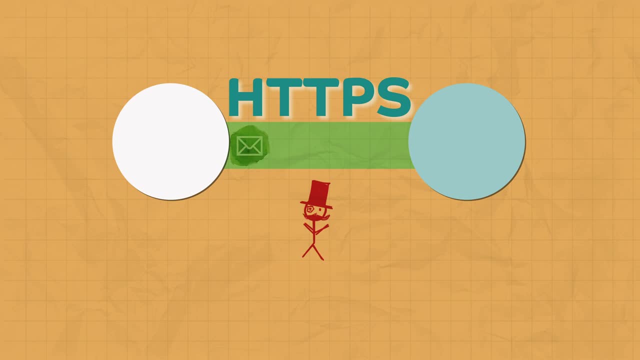 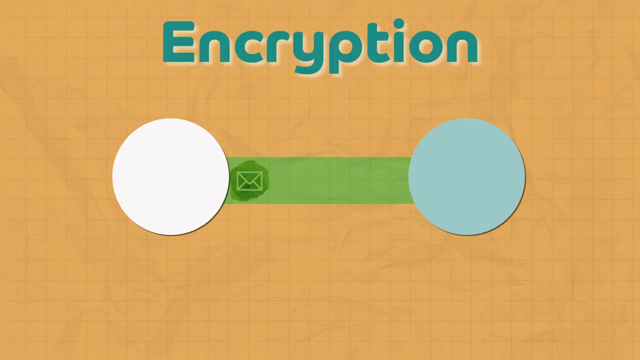 HTTPS for the connection to be secure. But before jumping into HTTPS and how it works, we have to define and understand what is encryption. Why should I understand this? Encryption is a key component to the secure aspect of HTTPS. Let's say a client is sending a simple message hello to the server and it doesn't want 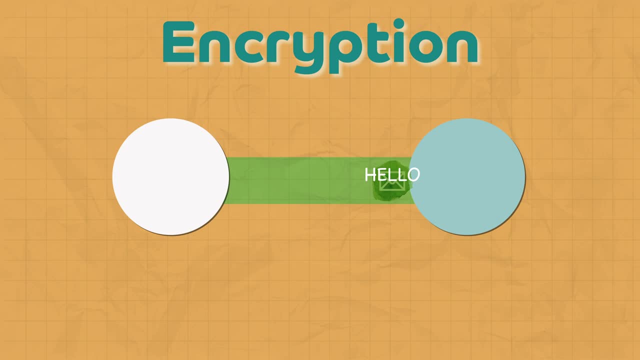 anybody else except for the server to read that message, and so we would somehow want to hide or obfuscate the message, and that is where encryption comes into play. The idea behind encryption is you somehow encrypt the message, meaning you turn it into a random string of characters. 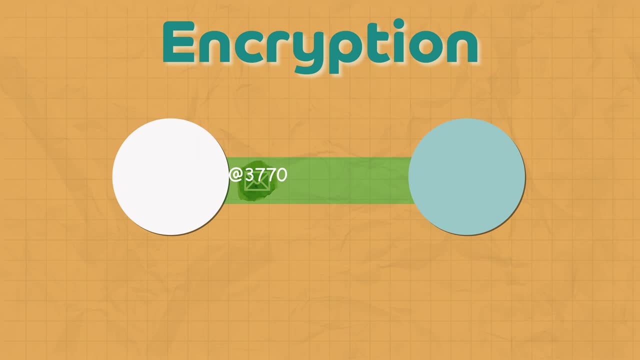 or some form of data that is no longer legible, and that the encrypted data should be able to be decrypted only by the particular party, in this case the server. So in this case, when the client sends hello, you encrypt it somehow into some random string that no one can understand, and then 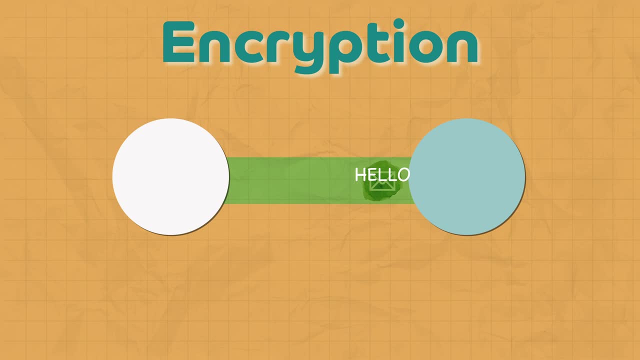 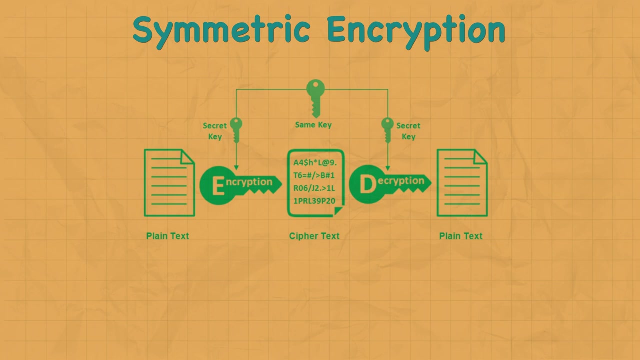 the server can decrypt that random string of characters and decrypting it would return an underlying message: hello. There are two types of encryption: symmetric encryption and asymmetric encryption. Let's look at them at high level. Symmetric encryption is an old and best known technique. 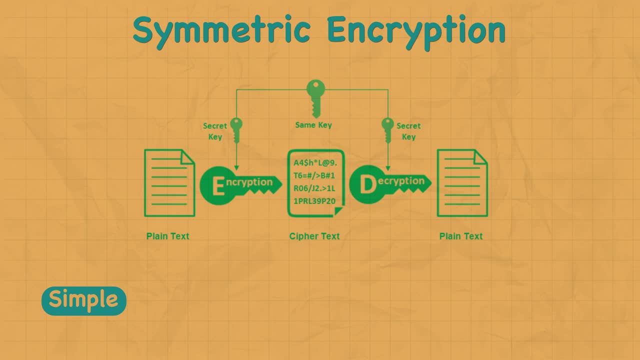 This is the simplest kind of encryption because it involves only one secret key to encrypt and decrypt information. You might think of a key as a secret, like a password used to encrypt and decrypt information. Symmetric encryption uses a secret key that can be either a number, a word or a string of random letters. It is often blended with a plain text of message. 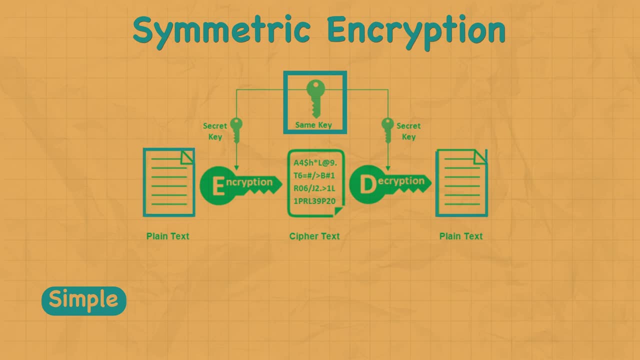 to change the content in a particular way. The sender and the recipient should know the secret key that is used to encrypt and decrypt all the messages. So imagine I got a key, say a string foobar, and then I use a special symmetric key algorithm using that key string foobar and the 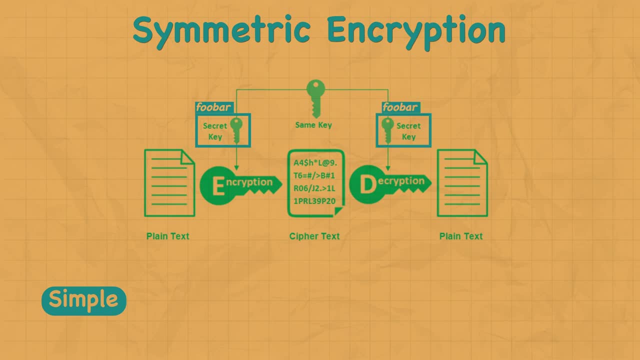 only way that data can be decrypted is using that key foobar. Generally, symmetric encryption uses AES or advanced encryption standard, which is a specification and describes a symmetric key algorithm that relies on single key. One nice thing about symmetric algorithm is that it is very fast because it relies on just one key, and the main disadvantage of the symmetric encryption- 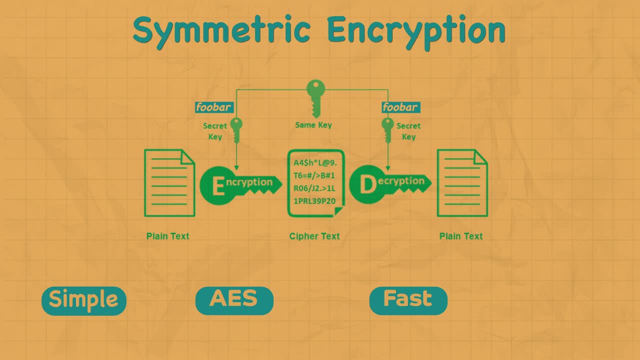 that is, all parties in the system. So if I want to encrypt a specific key, I need to decrypt it first. In our case, the client and the server have to exchange this key used to encrypt the data before they can decrypt it. This is usually fine when you want to communicate with a friend. 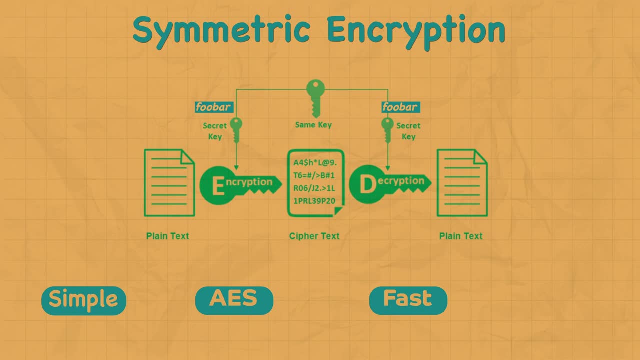 and you may just decide to share the key in person. But when it comes to client and server communication, how do the client and server establish a common key? That key has to be shared and in order to be shared, that key needs to be shared over security communications channel. 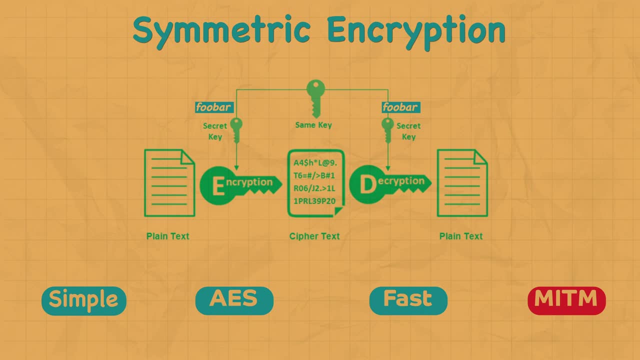 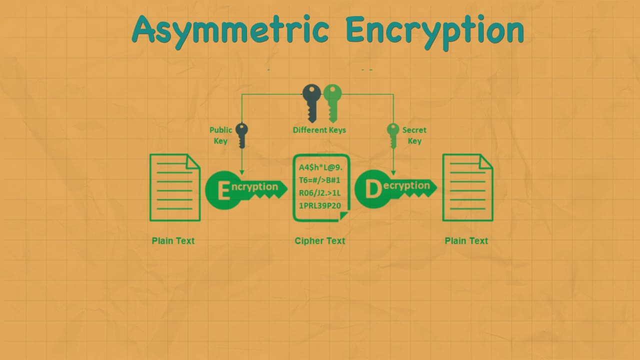 Otherwise, you can still end up with MITM or man in the middle attack. Okay, so now let's talk about Asymmetric Encryption. Asymmetric encryption is a relatively new method Compared to symmetric encryption. it uses two keys to encrypt information: A public key and a private key. A public key is made freely. 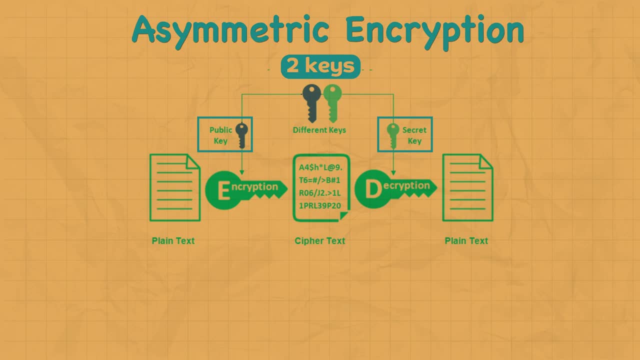 available to anyone who might want to send you a message, And the second private key is kept a secret so that you can only know. It is designed in such a way that a message that is encrypted using a public key can only be decrypted using a private key, While also 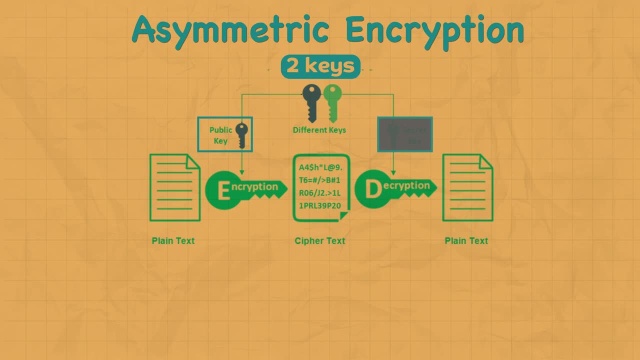 a message encrypted using a private key can be decrypted using a public key. As the name suggests, the security of the public key is not required because it is publicly available and can be passed over the internet. So, in our case, if a server has the private key, 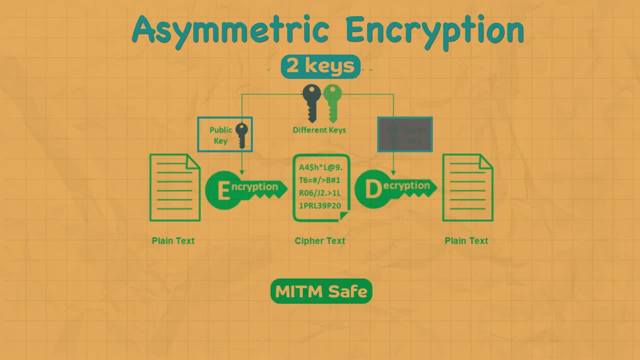 it would be the only entity to decrypt the messages of the client. Asymmetric encryption basically eliminates the need to share the key by using a pair of public private key, Which is why it is mostly used in our day-to-day communication channels, especially our 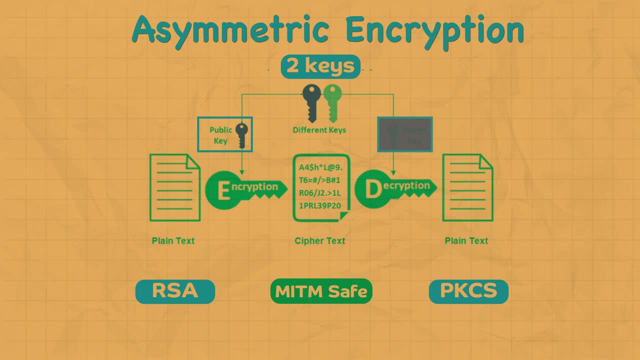 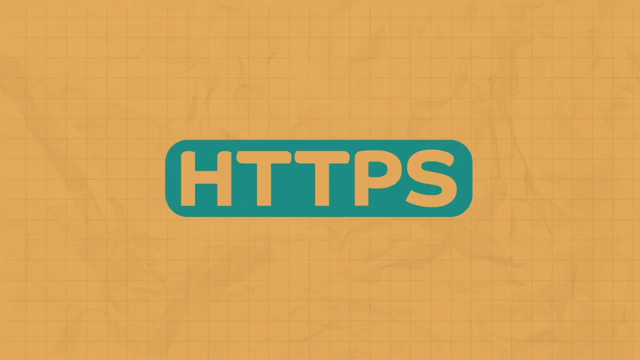 internet. RSA and PKCS are one of the popular asymmetric key encryption algorithms out there. Now this all brings us back to HTTPS, or how do we make HTTPS secure? Because, like I said, the S in HTTPS stands for secure. So here I am going to walk you through something known as 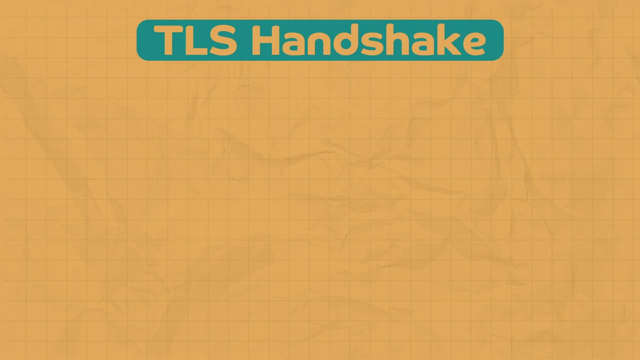 TLS handshake to understand how symmetric and asymmetric encryption come into play. And again, everything discussed here is at a high level, but at the same time, it will make sense in terms of system design interviews. So let's get started, Let's get started. Let's get started, Let's get. 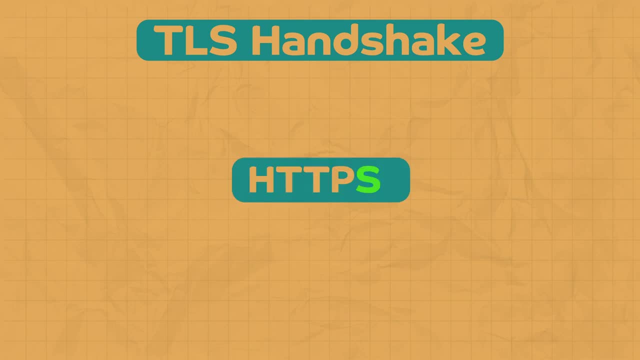 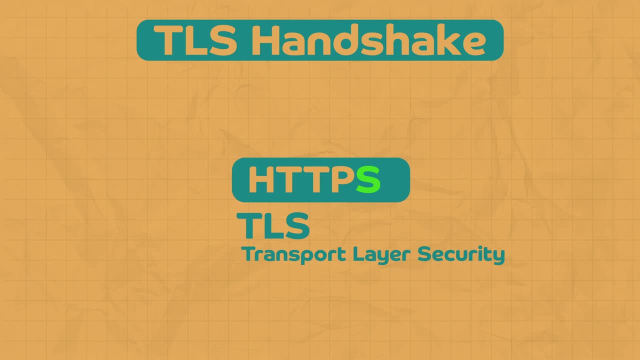 which is why sometimes you will hear HTTPS referred to as HTTP on top of TLS, Or in other words, HTTPS communication is encrypted using TLS And, by the way, the predecessor protocol to TLS was called SSL, which stands for Secured Circuit Layer. Today, we generally use SSL. 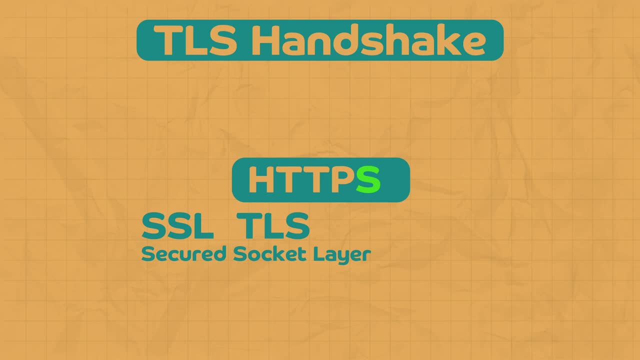 in the context of SSL certificates, which I will discuss shortly. Okay, so let's go back to our client and server example, But this time they are communicating over HTTPS And we need to understand what happens here. that makes the communication secure. In short, when the client and server establish a connection. 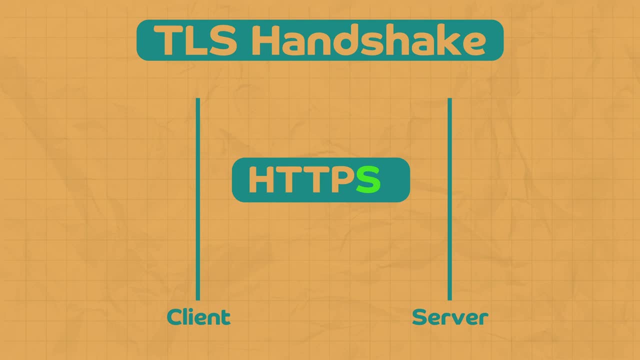 they first go through TLS handshake. This TLS handshake process establishes a secure connection. So what happens during a TLS handshake? First thing that happens is the client sends to the server something called as Client Hello or C Hello, which is a random string of Bytes. 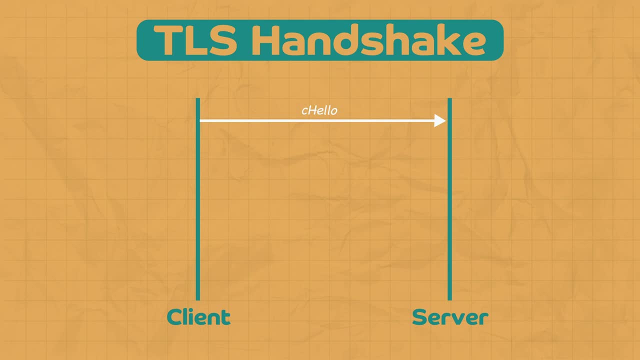 that the client generates randomly. And then the server responds to the client with two things. First of all, it responds with a Server Hello or S Hello, And it's just like Client Hello. It's a random string of Bytes generated by the server. 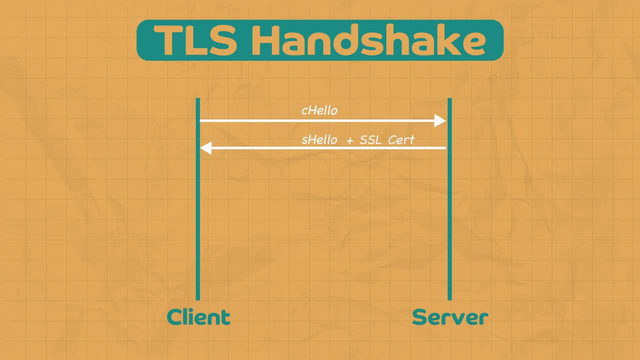 In addition, it sends the client an SSL certificate. Now we will get back into SSL certificate in a minute. for now, what you need to know is that in the SSL certificate there is a public key. So in SSL we need to know which different styles of keys of the server you want. 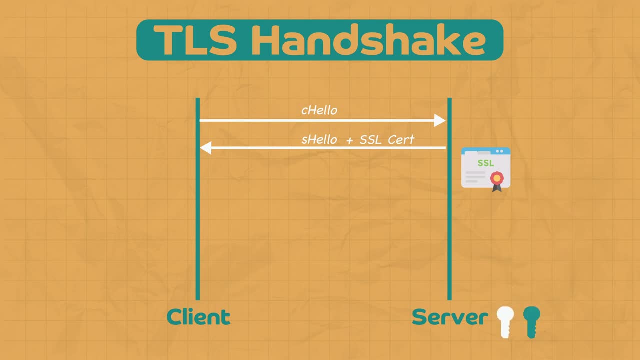 to something. So which way the serverGroup will communicate and what the serverinka will say will vary, Since we know that there are more earlierid days than here. the servergroup will essentially- which is coming from the public, private key pair the server has so say the server has a private. 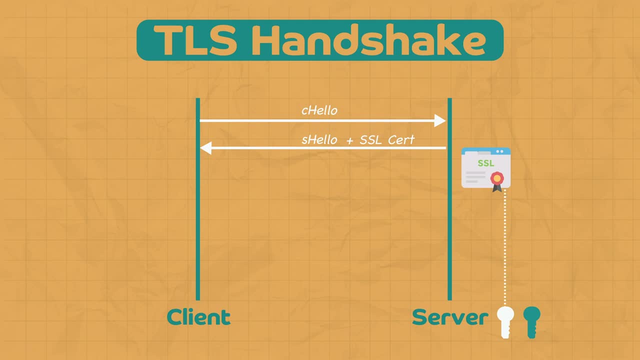 and public key here, and the server's public key is contained in this ssl certificate which is being sent to the client from the server. hello, now, once the client has the public key and using that, it generates another random string of bytes which we are calling here the pre-master secret. so when? 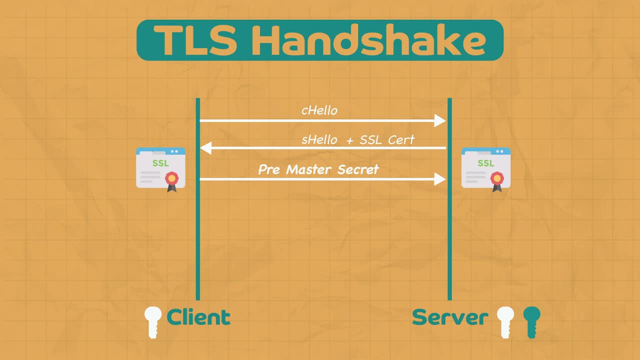 sending this pre-master secret to the server, it will encrypt this using the public key that it got from the ssl certificate provided by the server. when the server gets this client encrypted pre-master key, it can decrypt it because only it has the corresponding private key. portion of the 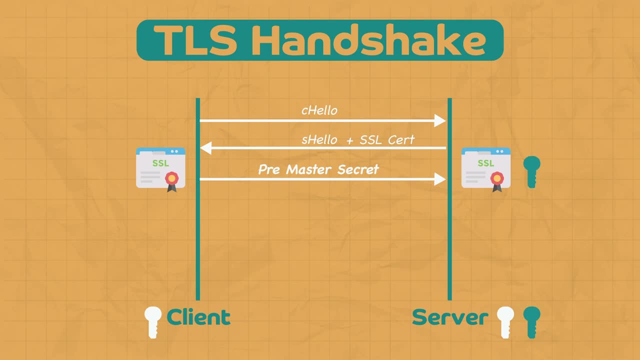 public key. at this point, both the client and server have access to three things. they have access to client hello, the server hello and the pre-master secret and using these three things, they are going to generate the session keys- actually four session keys, but in our case these details don't matter. 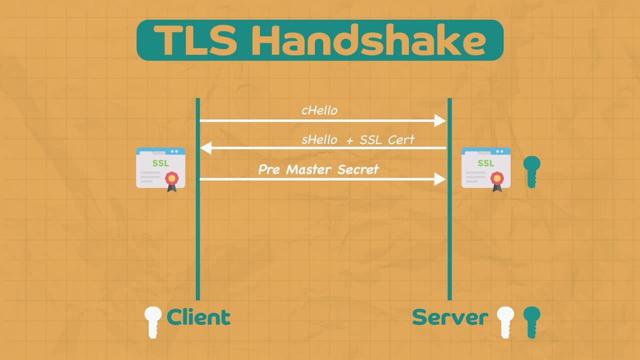 to us too much. what you need to understand is using these three things: the client and servers are generating four session keys. you can simplify this and, instead of calling four session key, you can say: the client and server are generating a symmetric encryption key for the session. this. 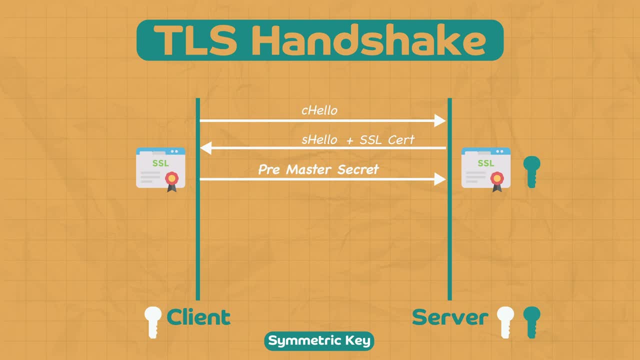 symmetric key is only valid for the session, and when the session is closed, the key is discarded, and this is done when you connect to any secure website where your web browser is the client which talks to the server of the website. at this point, there is still one thing we need to get clarity. 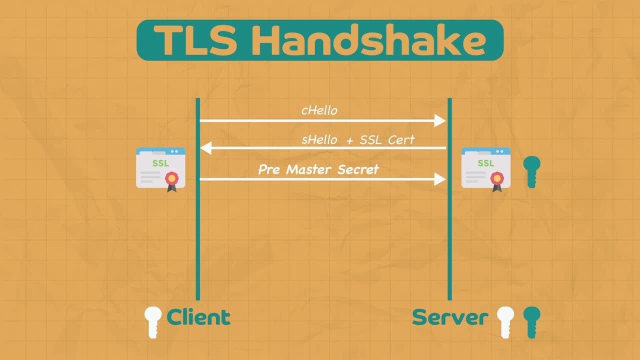 on, and that is ssl certificate. we saw that the ssl certificate has a public key, but then why don't we call it just public key? why call it ssl certificate? well, if the server just sent a public key here in the beginning, it is still vulnerable to mitm attack and a malicious actor. 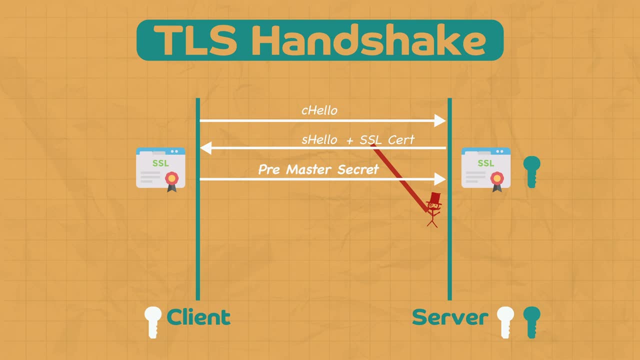 can interpret that initial communication and modify the public key so the client might end up having the public key of malicious actor and it will encrypt the pre-master secret using the public key of the malicious actor. the malicious actor can then be able to decrypt the pre-master. 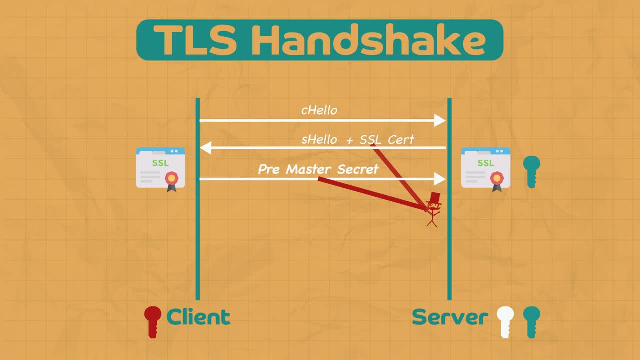 secret and basically the entire communication channel is hacked. at this point, the problem here is how the client knows the public key that comes from the server is off the server, in other words, how the client can trust the server, who the server claims it is. this is where ssl certificates come. 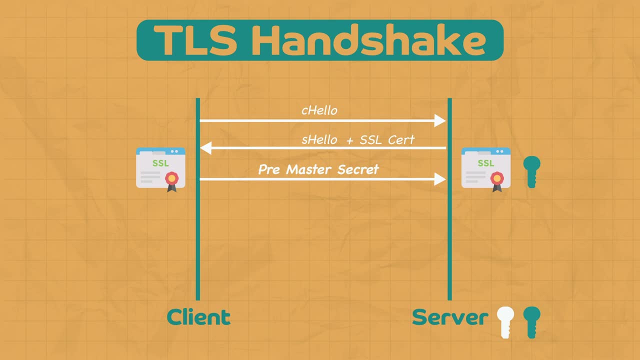 into play. ssl certificates are granted by trusted third party called the certification authority, or, in short, ca. a certification authority, or ca, is a trusted organization that verifies websites and other entities so that you know who you are communicating with online. the certification authority can be non-profit or for-profit organizations, such as let's encrypt or digi. 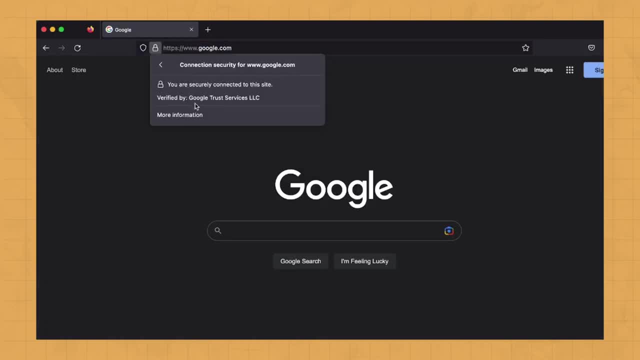 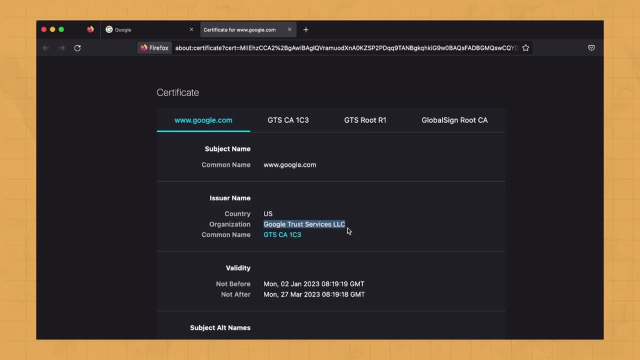 cert. if you type googlecom in the browser, with few clicks you would be able to see certificate authority. the certificate issued by the certification authority is a digital item. it contains the public key of the server. it also contains the name of the entity that owns this public key. that is, the server name. 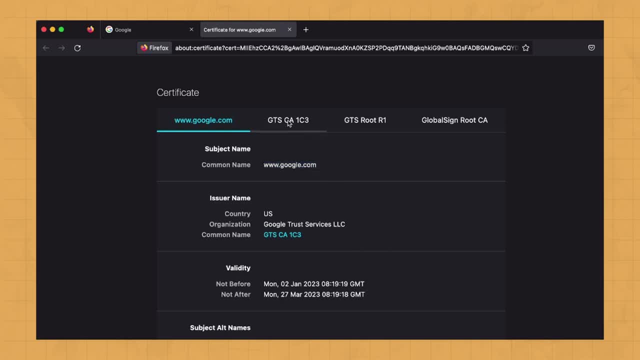 and some sort of assurance that i am a trusted third party and the certificate authority and i am assuring that this public key belongs to this server and this ssl certificates prove that this server is who they say they are. now this: all information will be signed by the private key of. 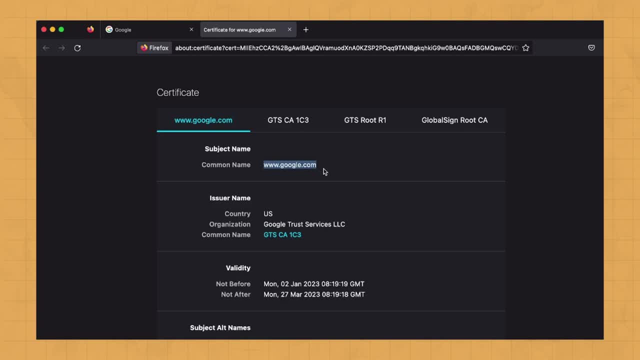 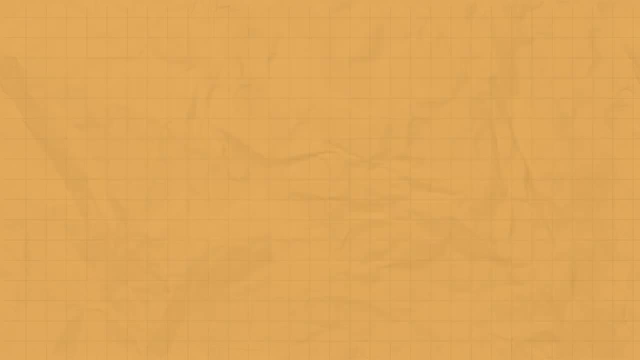 the certificate authority itself and the client in order to verify this digital signature. the client will be able to verify this digital signature and the client will be able to verify this digital signature, and the client will use the public key of the certificate authority to clarify. we have talked about two public key- private key pairs here. one public key, private. 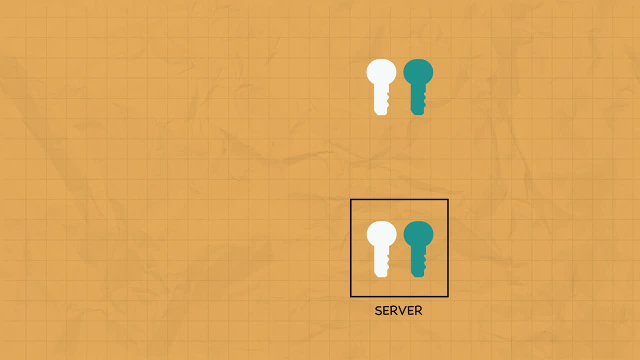 key pair is of the server we discussed earlier. here we are talking about the public key- private key pair of the certification authority itself. the certificate is signed by certification authority's private key and the fidelity of the certificate can be verified by the client or by any client just by using the public key of the certificate authority. 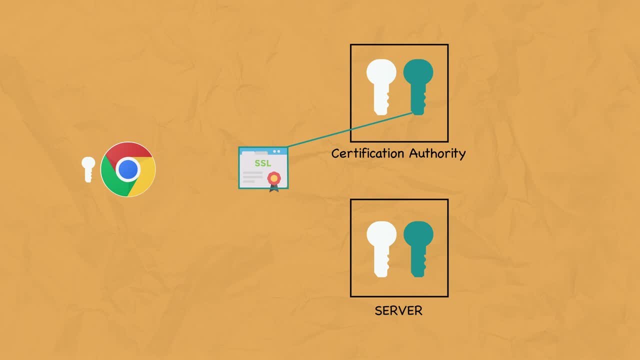 and And since these certificate authorities are well-known trusted third parties, most browsers such as Google Chrome or Firefox that we use will already have the public key of all these trusted third party certificate authorities stored, such that it can verify all the certificates the browser will be getting from various websites. 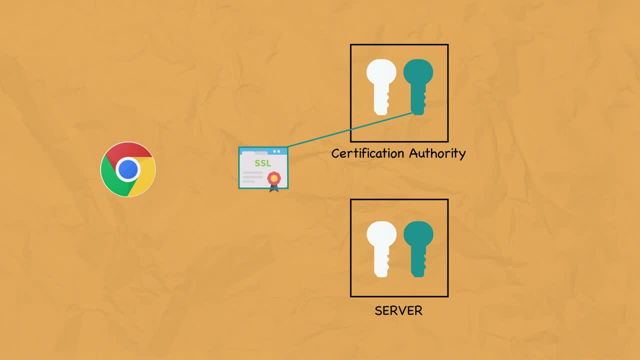 So when you type a URL on the server, if the site is not running on HTTPS, Chrome or any modern day browser will flag that website as insecure. Since we have been talking about so many keys, things can get really complex, So here I would like to reiterate the entire TLS handshake one last time. 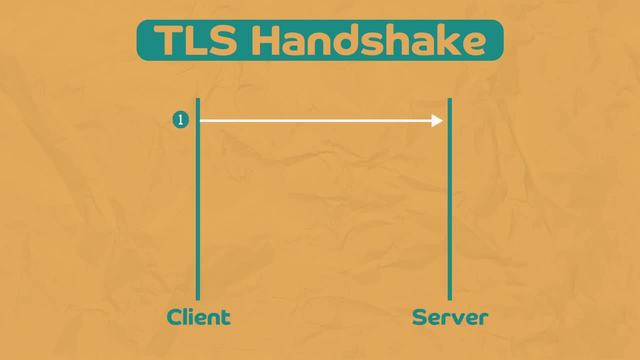 So let's begin. The client or your browser sends a message to the browser client hello. The server responds with server hello, as well as its SSL certificate, which contains its public key information about itself and is digitally signed by the certification authority using the certification authority's private key. 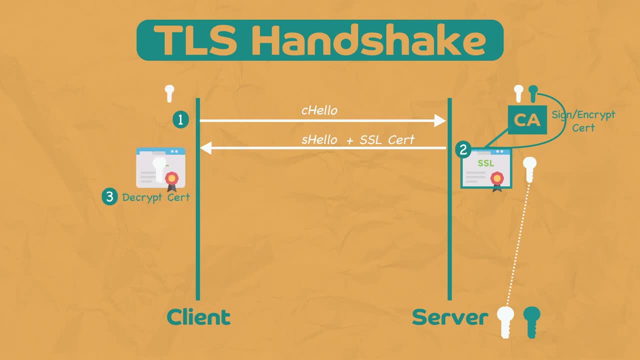 Then the client or browser very ifies by decrypting the certificate using the corresponding public key of the certification authority. It then gets the public key of the server from the certificate And, because it was digitally signed by the certificate authority, it is now being assured. 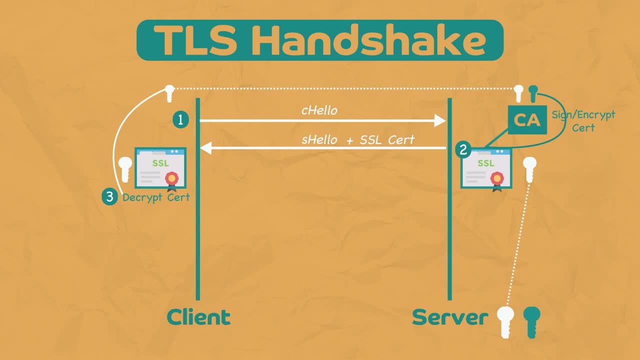 that the certificate belongs to the server. The client then encrypts the premaster secret using the public key of the server, sends it back to the server, And then the client and the server use the client, hello, server, hello and the premaster. 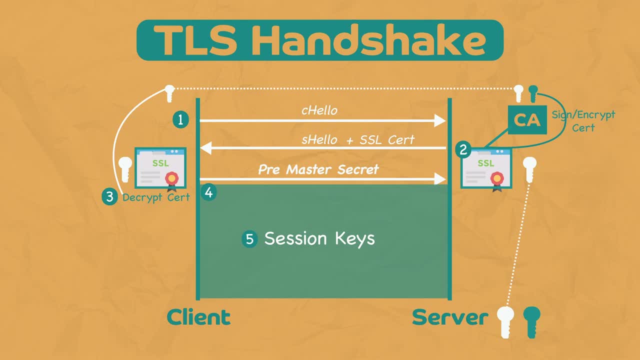 key- And this is how HTTPS works- to generate session keys, which will then be used to symmetrically encrypt any further communication between themselves. And once the connection ends, the session keys are discarded. They are only valid for the session and any future connection will go through this entire. 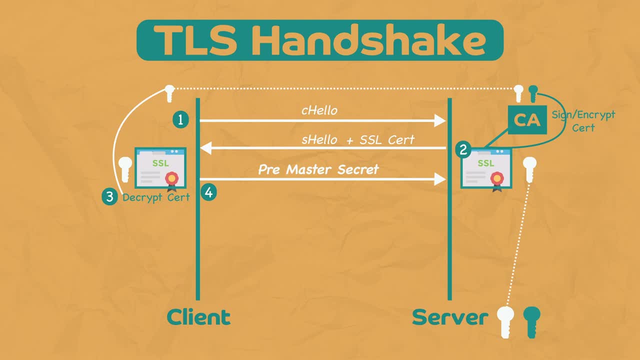 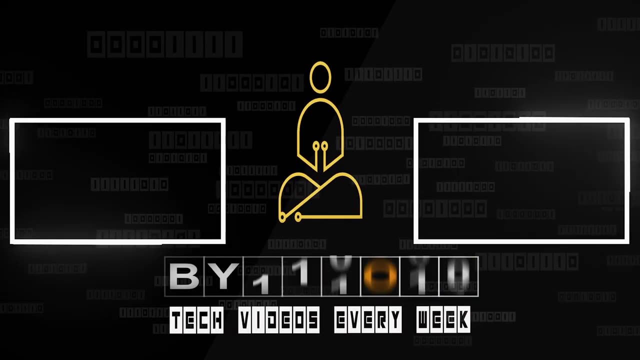 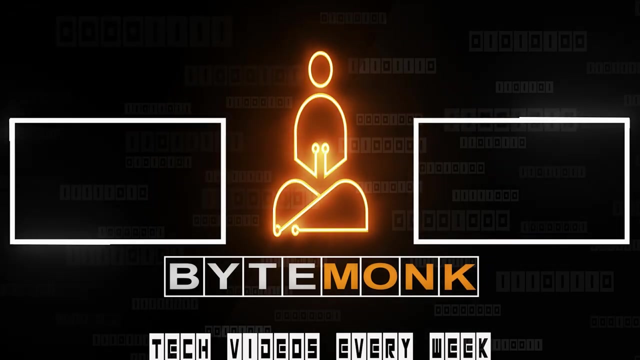 process of TLS handshake And this is how a client and server establish a secure connection over the network. and this is how HTTPS works and modern day systems handle security. Thank you for watching.